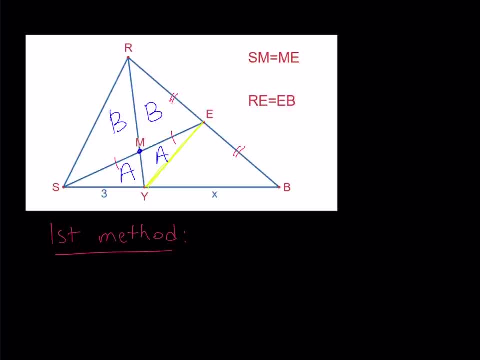 first thing I'd like to do. And then, of course, I want to be able to write everything in terms of A and B using the other relationships. Notice that RE equals EB. That means that the area of REY and B is in the middle, So this is also A plus B. So I'm adding A plus B and that gives me A plus B. 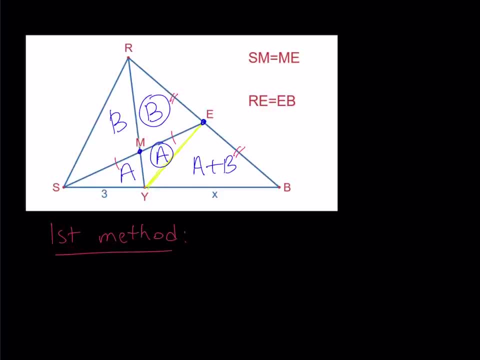 because E is a midpoint. Hopefully that makes sense Great. So this area method is actually very helpful with these kinds of problems where ratios of you know segments are asked, especially this type of problem. So let's go ahead and see how we can use this Now. 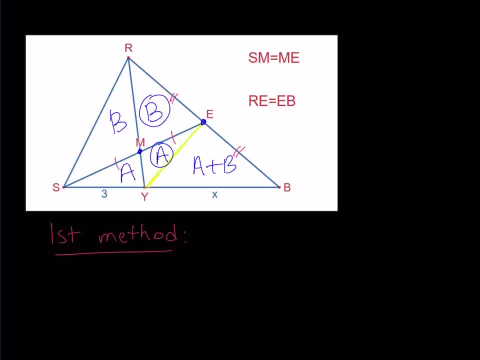 I want to focus on triangle SRB, And in triangle SRB I want to focus basically at this point, because that's where my 3 and X are separated. So here's what I'd like to do. I want to focus on two triangles here, actually RSE and RYB. So what is that supposed to mean? Well, 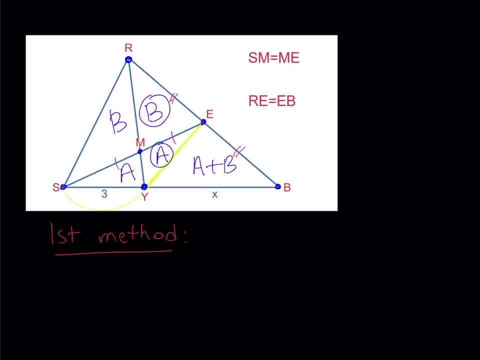 they don't have the same area, but if you look at their bases, the bases are 3 and X. So what is that supposed to mean? You have two triangles and you know that their basis is like, let's say something like A and B, And let's call: this area is S1 and this area is S2.. These two triangles, 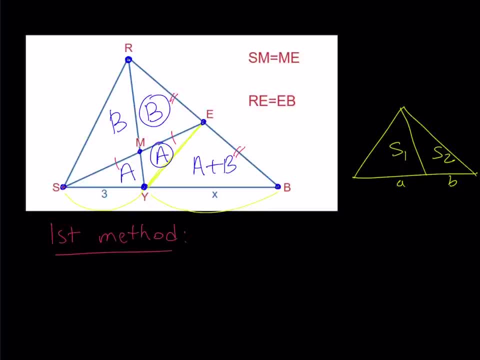 have the same area. So what is that supposed to mean? Well, if you look at their bases, the same area- I mean- sorry, not the same area- the same height. Therefore, the ratio of their areas is the ratio of their bases. In other words, S1 over S2 is the same as A over B. That's what. 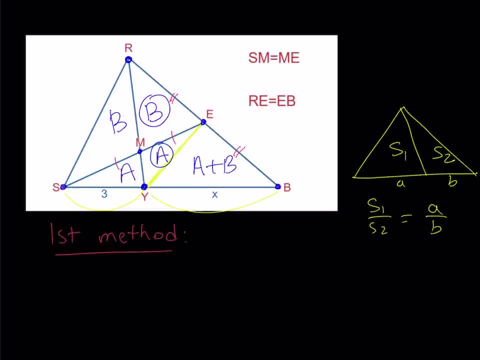 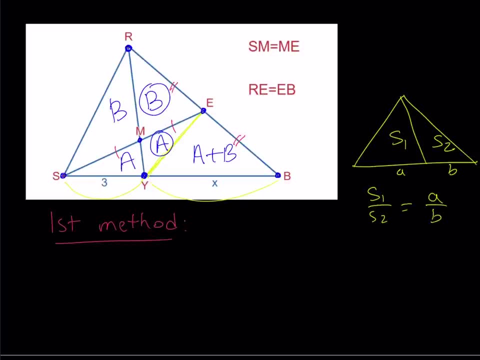 we use to find AA and BB here- Same idea, but the areas were equal in that case. So now, looking at the big picture, I noticed that the area of SRY is A plus B, So I'm going to compare that to the. 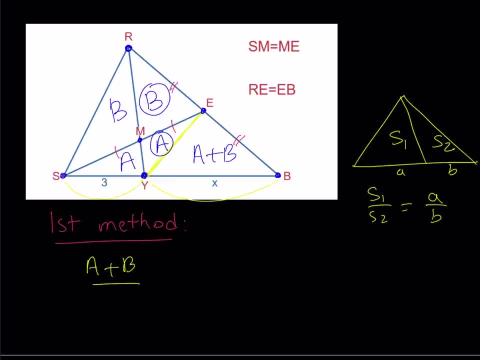 area of RYB And that is going to be 2A plus 2B. All right, Yay, I can finally say 2B or not 2B, Okay, And that ratio is equal to 3 over. 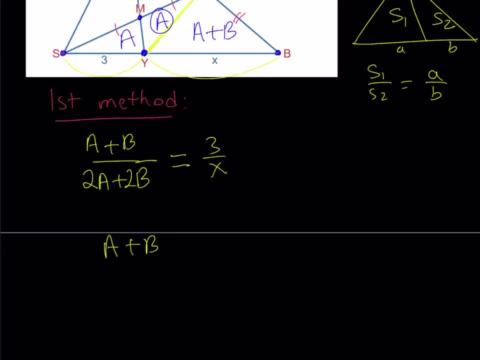 X, But notice that we can take out a 2 here and simplify this, And this gives me one half. So from here I get: X equals 6 and X is what I was looking for. X is the unknown right- Great, So. 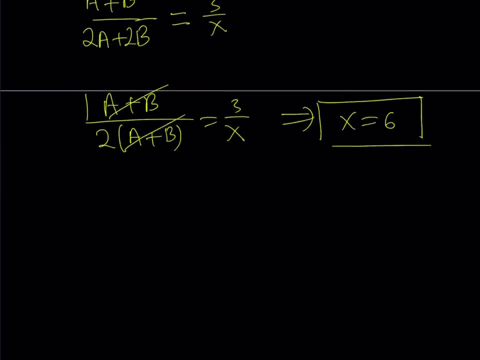 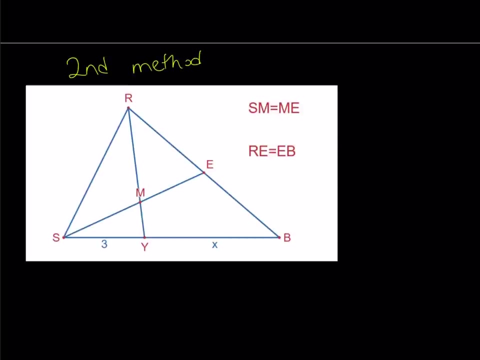 this concludes the first method. Let's go ahead and talk about the second method. Now, what is my second method involved? Let's do this here, because I have another picture. So the second method involves what's called mass points. I hope you are familiar with that, If not, 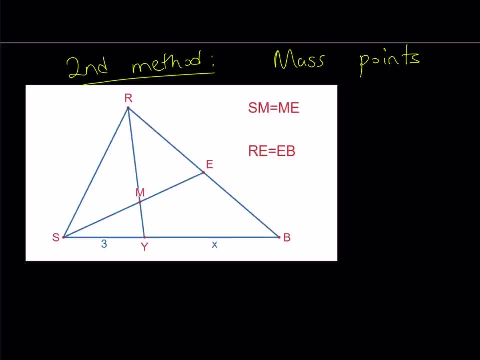 please Google it and take a look, because it's a really cool topic in geometry. So mass points basically tells us that, okay, we can just assign weights to the vertices, And here's the rule that we need to follow when we're assigning weights: Okay, We always have to make sure that weight 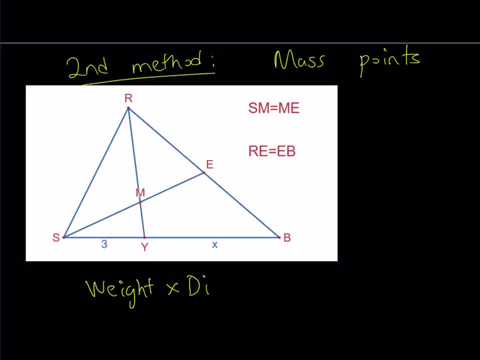 one times distance equals weight two times distance. So weight times distance is going to be fixed on a line segment. We're going to start by assigning weights to each vertex, as we're going to start at the outer vertices. And then here's another rule: When you have a segment like RB. 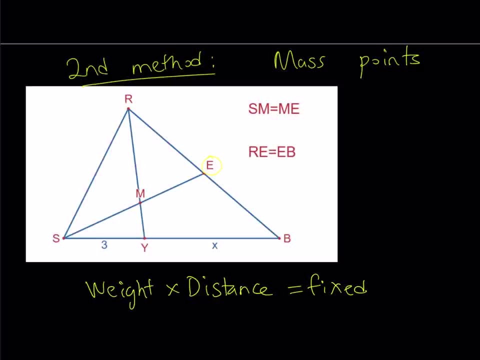 and we know that E is on RB. E is in the middle, basically not necessarily right in the middle. It is, but it doesn't always have to be that way. That means that the weight at R and B will be added And you're just going to assume that all the weight is. 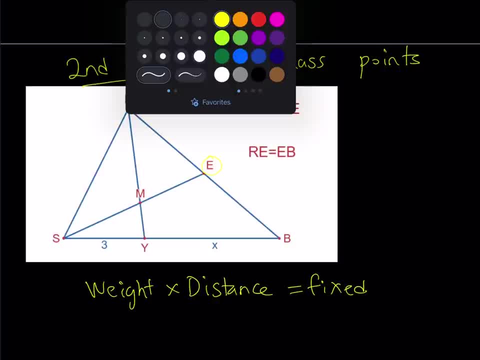 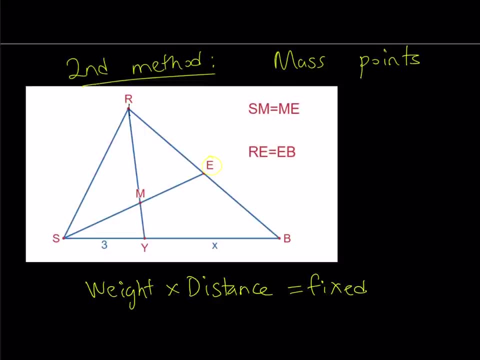 accumulated at E. Let me go ahead and clarify what I mean by this, by assigning weights, because that's the best way to understand it. So let's go ahead and start by assigning a weight of one. And, by the way, for assigning weights you don't have to use any specific number. 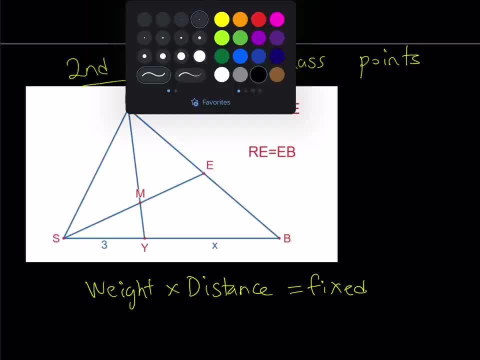 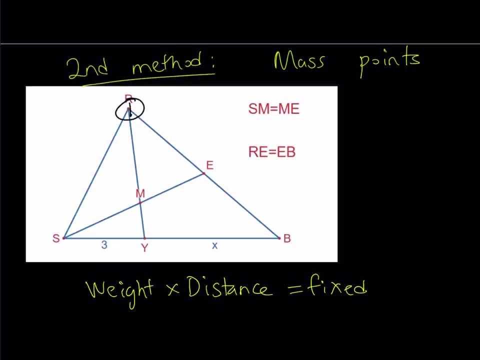 because what matters is the ratios. So the only thing that matters here is the ratios. As long as you keep that constant, that's good. So let's suppose this is a weight of one and this is a weight of one. Now how could I assign the same weights? I can, because E is a 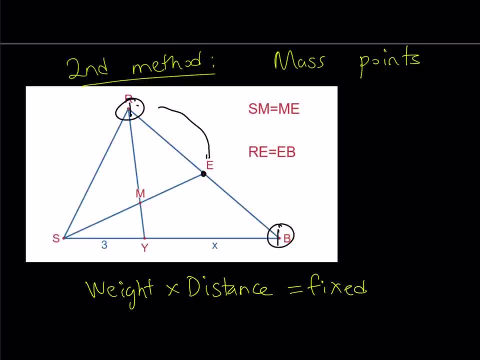 midpoint. So the weight times the distance here is going to be the weight times the distance. Since the distances are equal, the weights are equal. Does that make sense? I hope that makes sense. The formula says weight times distance always have to be fixed on that same line segment. Great So. 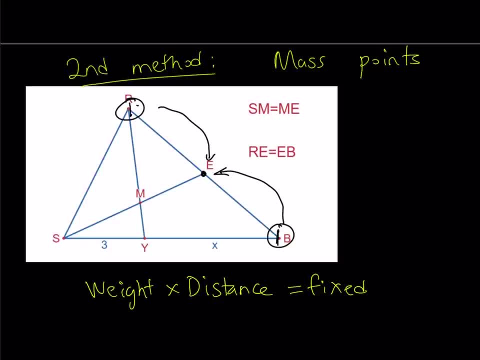 that means that the weights are equal at these two vertices. Great, And what is our next rule? The next rule is you're supposed to add the weights to get the cumulative weight or whatever accumulated weight. So in this case that will be a two. Okay, So at E I have a weight of two. Great, Awesome. Now. 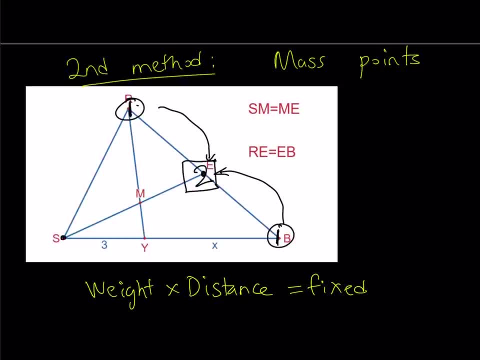 here's the thing. From this point I can go to S. Notice that SM equals SME. Therefore, M is a midpoint, which means that if I assign a weight of two for E, then I also have the same type of weight for S. So that means I have a weight of two for E. So that means I have a weight of two for E. 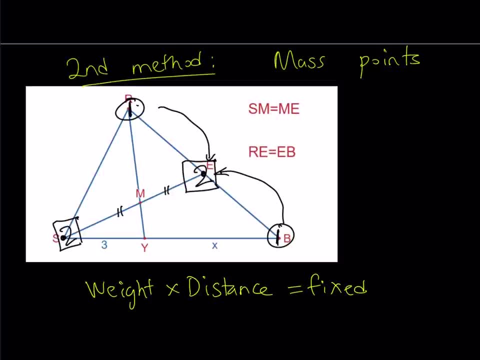 Awesome. And that tells you what. Two plus two equals four, So the weight at M is supposed to be four. Let's go ahead and use a circle for that. If you want, you can use a different shape, Doesn't really matter, as long as you know what you're doing. Now this tells me something else, Notice. 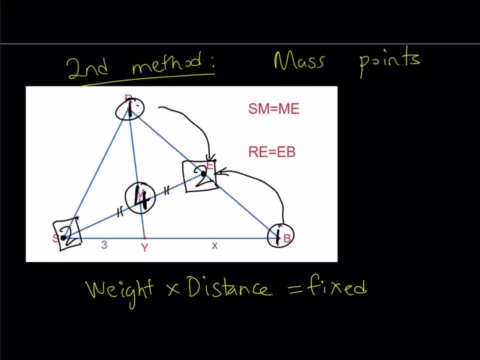 that how I can transition from one segment to the other by using the weight relationships. Notice that here I have a weight of one and here I have a weight of four. So what does that tell you about the weight at Y? Because the sum of the weight of one and the weight of the other is the same. So 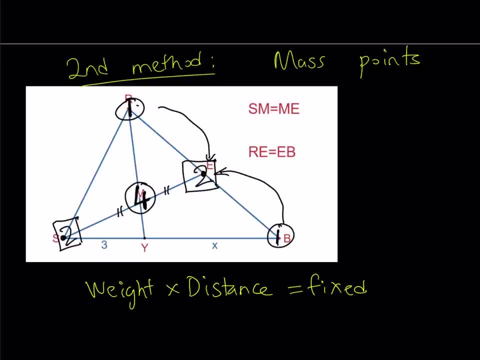 the sum at weights R and Y needs to equal four. Four minus one equals three. In other words, this is supposed to be a weight of three, And this is the most critical part, because that tells you what. Well, here's the thing. I considered different segments and I was looking. 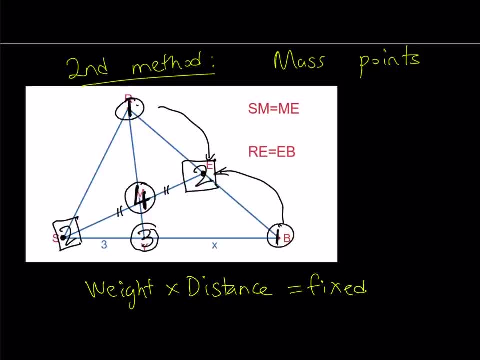 at RY, And on RY I noticed that the weight at Y has to be three, because three plus one equals four. Makes sense, right? It's basic arithmetic. You're basically adding, subtracting numbers, But that tells you more than this, because if you look at this carefully, 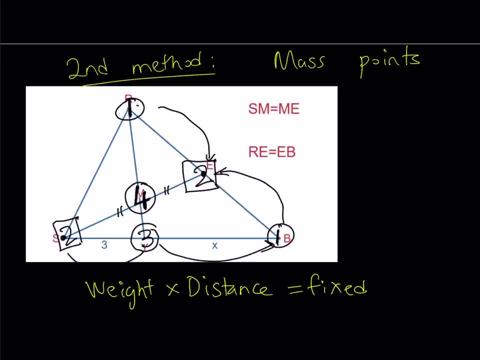 here we have another relationship right On SB. I have point Y, since point Y is shared, and I have all the weights: Weight. What is that supposed to mean? Well, it just means that you can find the ratio of the side lengths, because what's our rule? Weight times, distance.